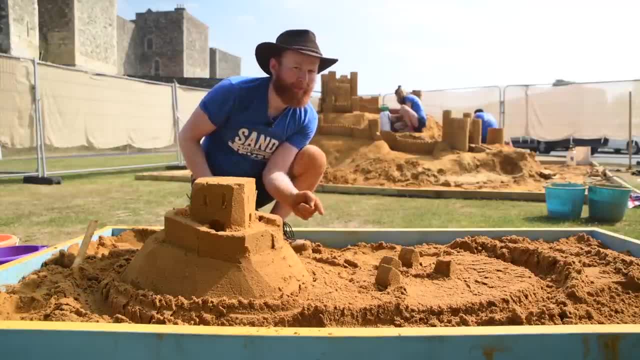 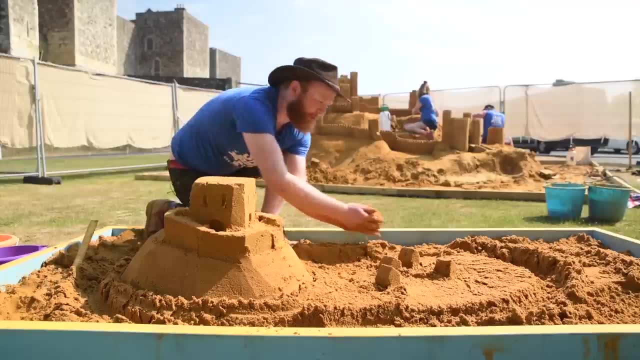 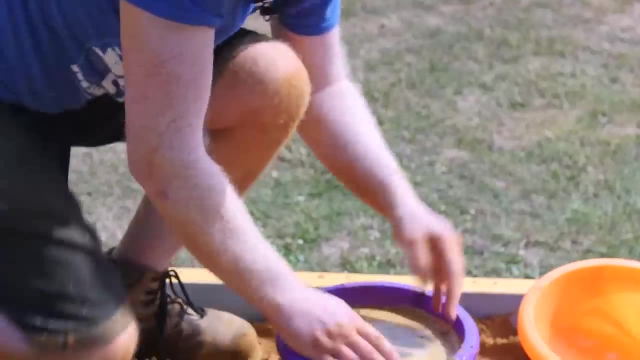 even got a little village, but we've got no walls to defend it. so tip number five is to make walls. You push the sand together and pinch down with your thumb and then just take the sand and give it a little finger tap, just like that. and when it stops being like jelly, then 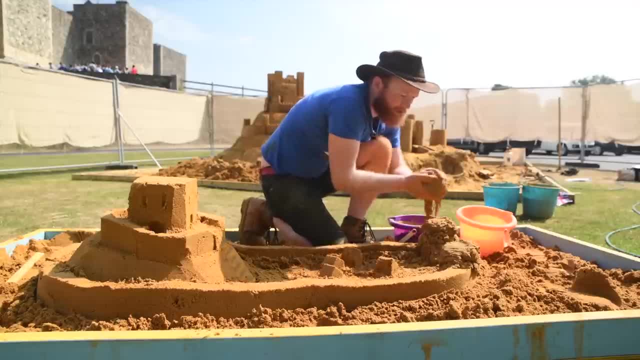 you stop tapping and you'll start to make these towers. Oh, you've got to be kidding me. It's so nice and gooey. Look at that. So here we have our sand castle, and it's got its walls, but it's got nothing to hide behind. 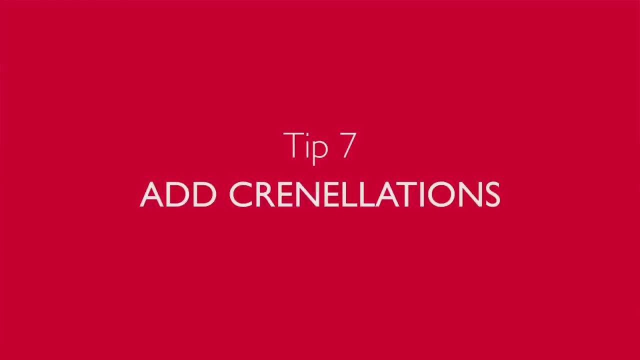 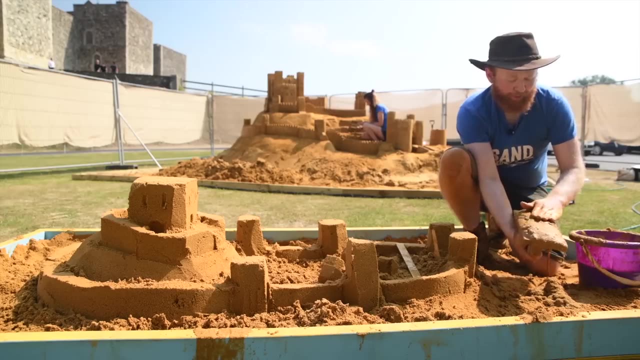 for the soldiers to protect themselves. Tip number seven is to make cremelations, and for this you're going to need a wooden float and plenty of muddy sand. So get your muddy sand and put it onto your wooden float and give it a little finger tap. 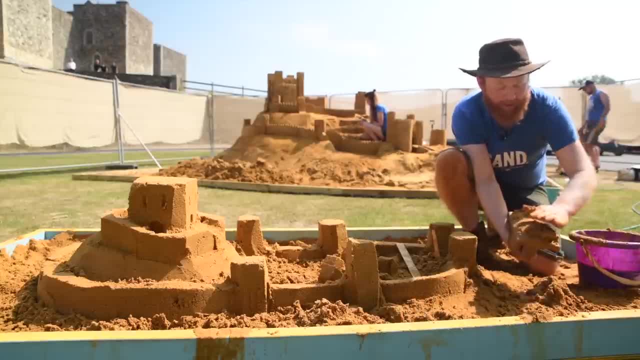 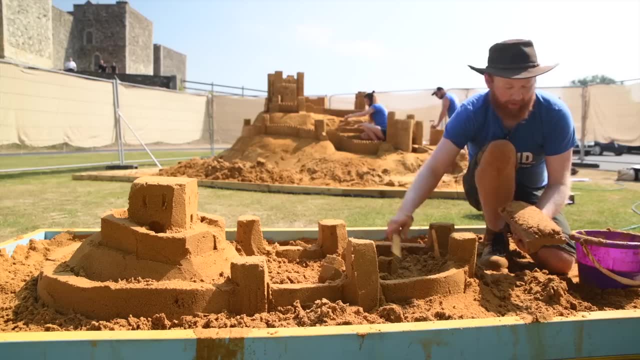 again to vibrate the sand and then, if it's too muddy, just add a little bit of dry sand and keep going until it basically turns into a hard piece of sand. You'll then take your ruler and you'll make a little bit of sand. 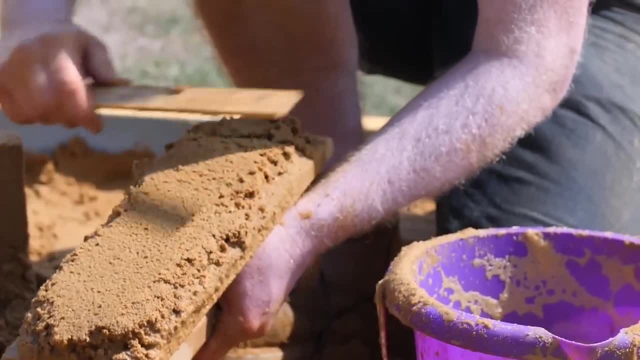 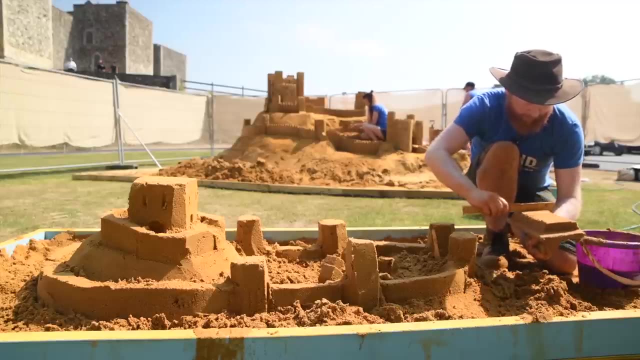 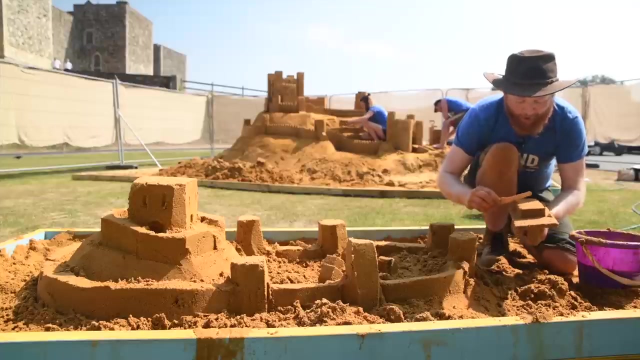 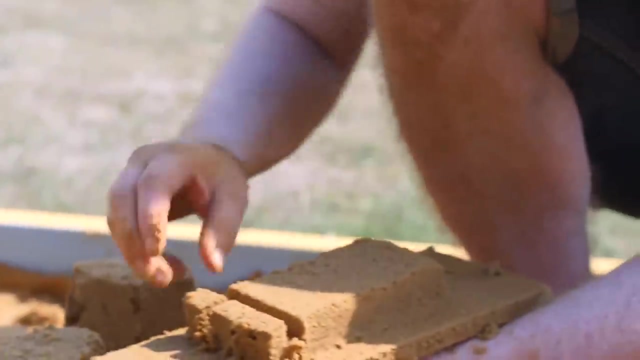 When you've got your chocolate bar, you need to cut it up into little blocks, Gently take them over and put them onto your towers. So you've got your chocolate bar and you need to cut it up into little blocks and gently take them over and put them onto your towers. 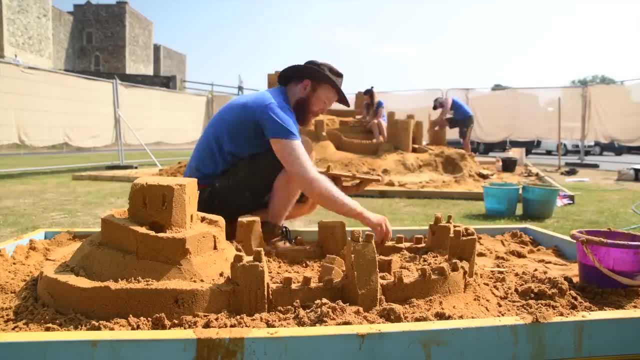 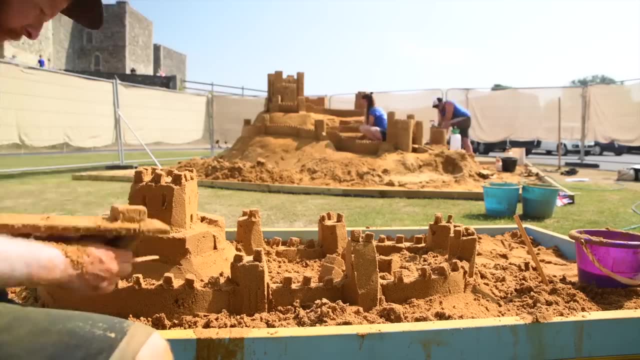 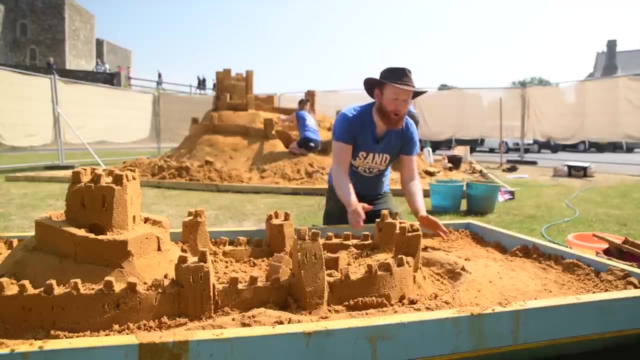 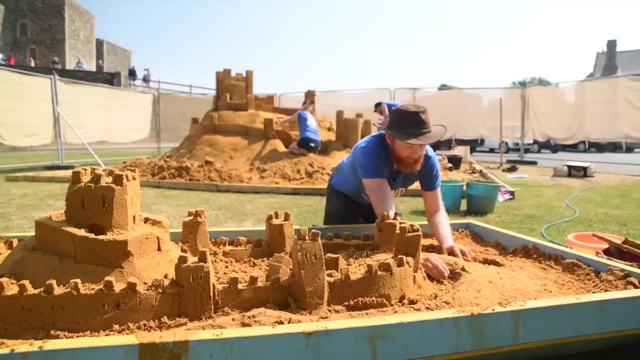 Gently take them over and put them onto your towers. Okay, so we have our castle and we have our moat, but we have no way of getting out. So tip number eight is to make a drawbridge. So what you do is you just make your hand nice and big like this and have it really. 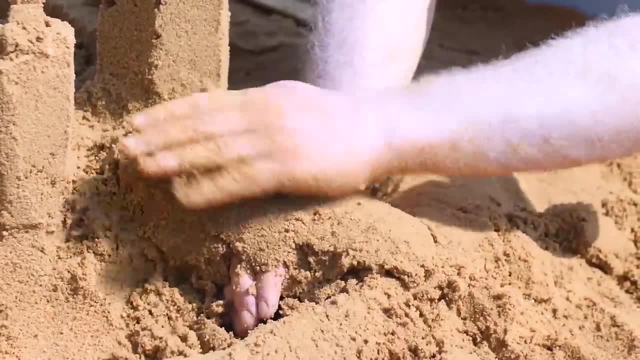 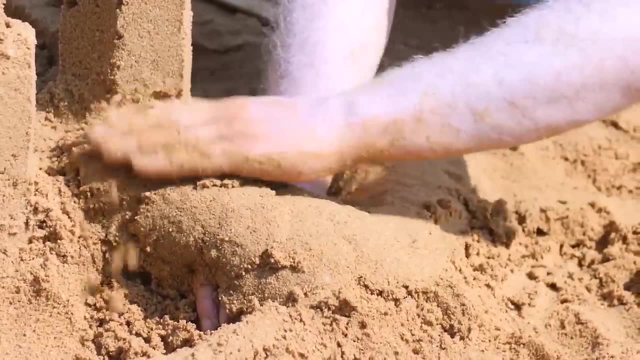 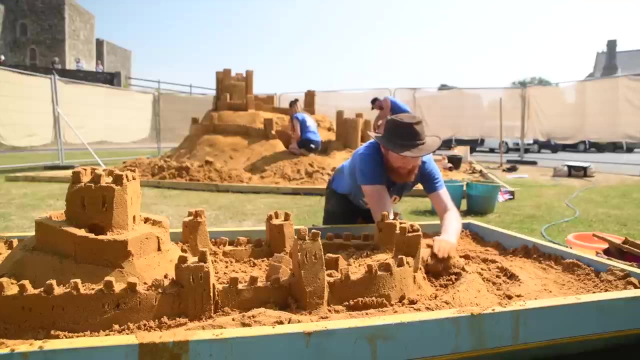 grazed a little bit and then just pat the sand over it like so, And then I'm just going to take my hand down and make it smaller and hopefully I'll be able to take my hand out and there'll be a little problem after that.